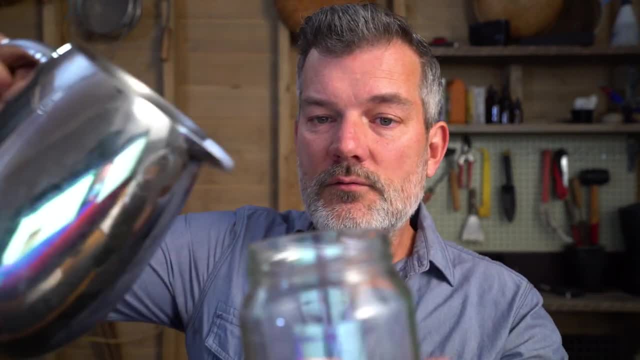 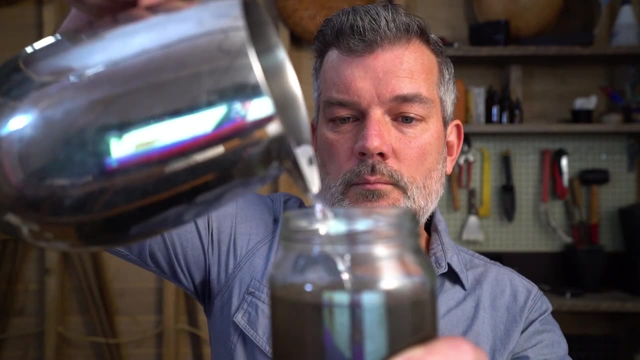 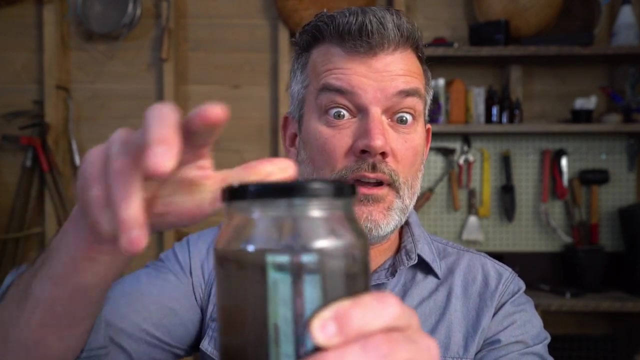 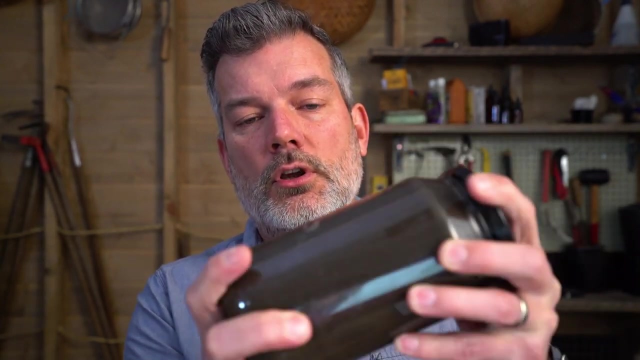 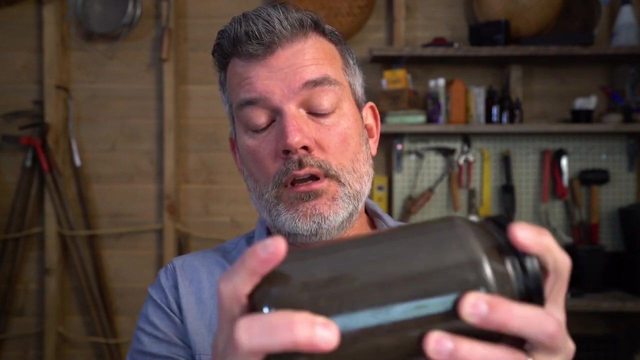 Just washing up liquid And then fill your jar 90% up with water, Almost to the top, Put your lid on tight, Make sure it's tight, And then we want to shake it. Give it a really, really good shake. That dishwashing detergent just helps. all the dirt get saturated by the 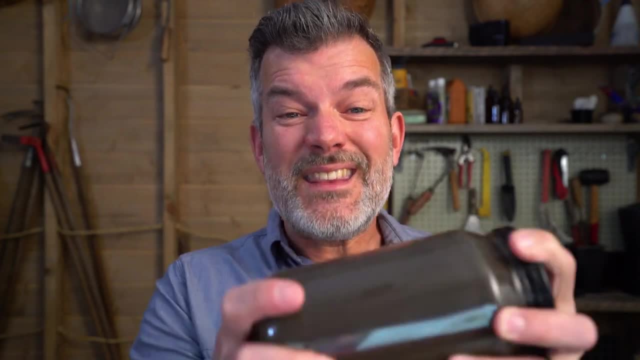 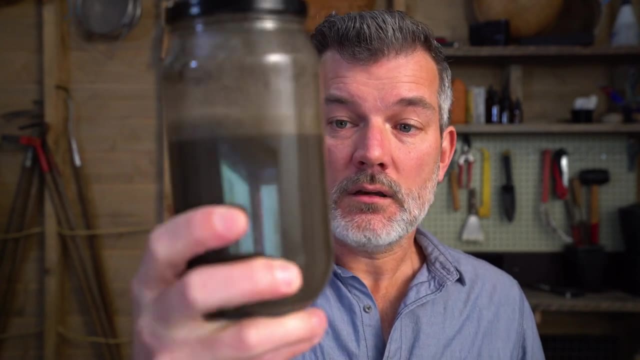 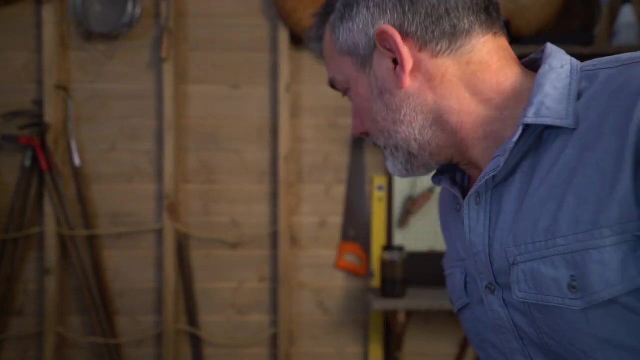 water. You want to shake that for at least three minutes And then you can't see anything. You've got to let it stand overnight for those particles to settle out. So I've got one that I've done previously just over here. 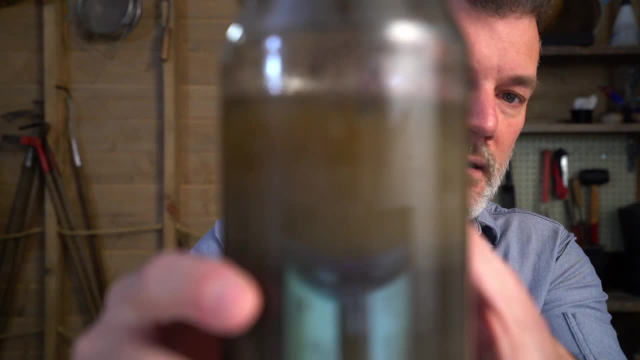 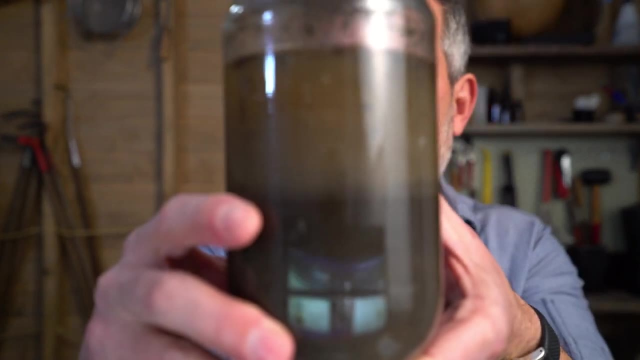 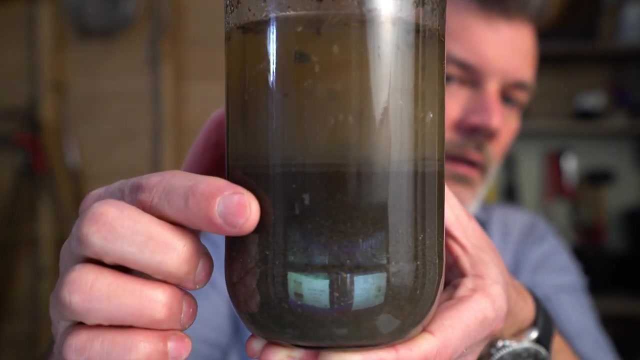 And what you should be able to see in that is that all the different particles have started to settle out. Oh, camera comes into focus And we've got the water floats on the top, and then we've got the sand at the bottom and the silt in the middle. 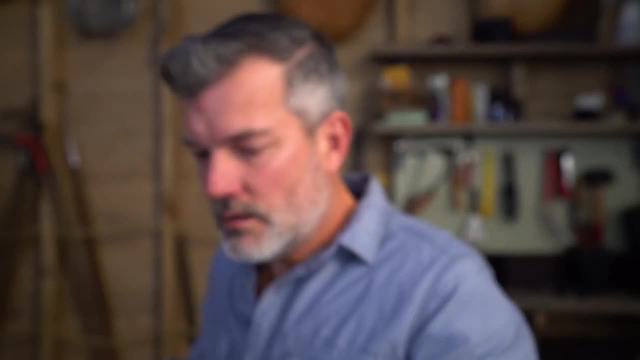 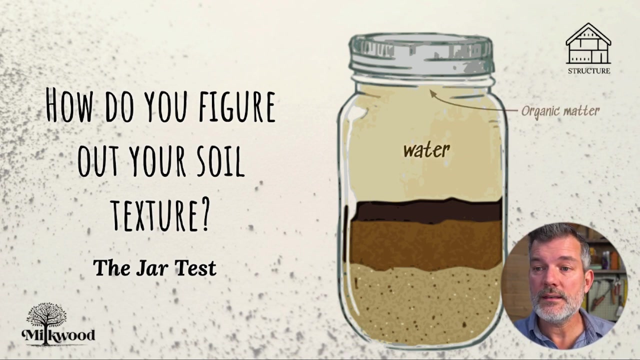 and the clay up there. So I've got a diagram to make that a little easier to see. So the first thing is the jar's full of water and the organic matter will float all the way to the top. Then the first thing to settle out, because it's the largest, heaviest particles. 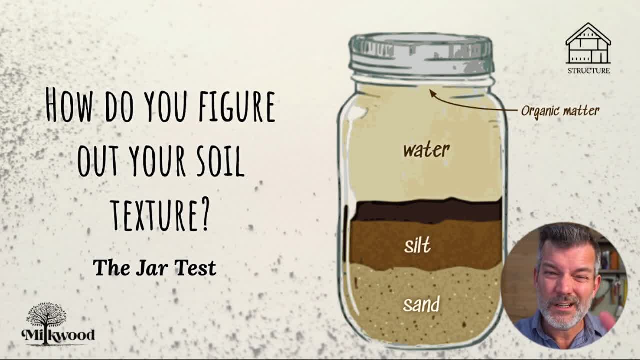 is the sand, Then the silt settles out, you know, in the first sort of 10 minutes or so, And finally the clay takes ages to settle. It might take a day or so for it to all settle on the surface and you get back to reasonably clear water. 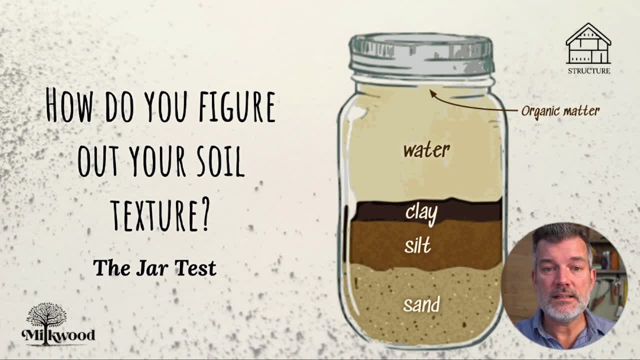 So what you need to do then, once it's all settled like that, is you need to get yourself a ruler like this one and measure the different heights of those different materials. So in this case I made it a little simple. for our example, You can see there. 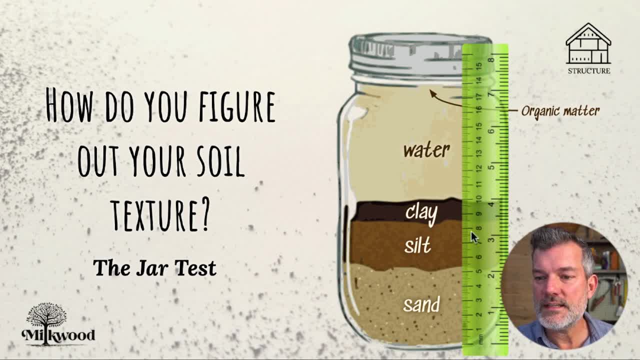 there's about 100 millimetres, 10 centimetres or 100 millimetres of total solids from here, the bottom of the jar to the top of the clay, And if we measure the sand we've got about. 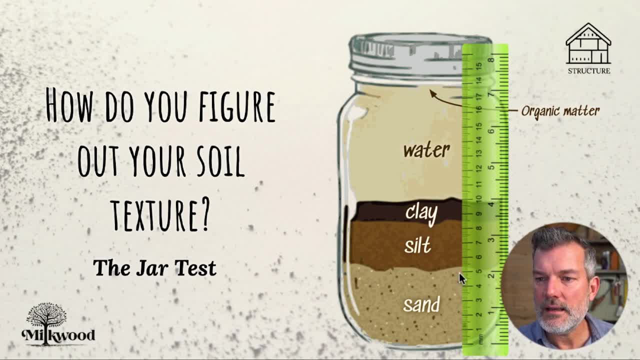 50 millimetres of sand and you might be able to see there that clay. we've got about 15 millimetres of clay, So that makes it really easy. Fifty percent sand and 15 percent clay, So the rest is. 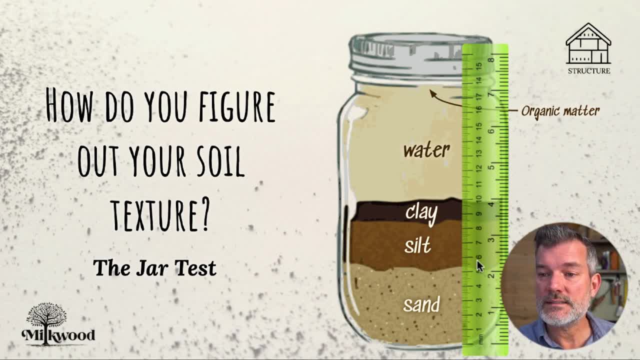 silt, So you don't even need to measure that. That's 50 plus 15 is 65, and that leaves- oh no, yep, 65,, which leaves 35 millimetres of silt. So that makes it 50% sand, 15% clay and the rest. 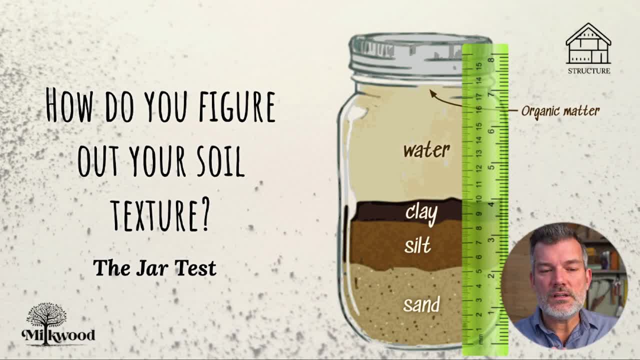 about 35% is silt. It's those ratios that determine your soil texture. When you hear gardeners talking about a clay soil or a sand soil, they're talking about soil conditions. So, or a sandy loam, that's what they're talking about. 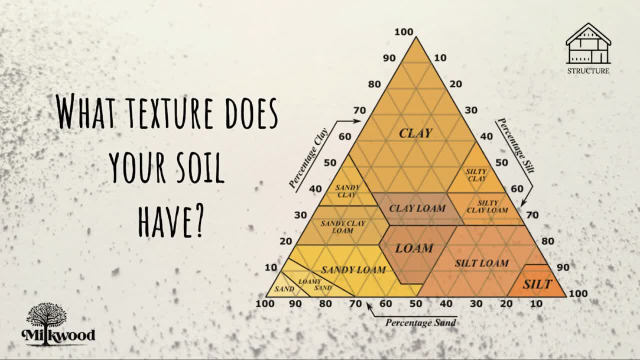 Now this beautiful thing is the soil pyramid, an amazing little triangle plot chart that was developed nearly a hundred years ago, way back in 1927, by two scientists called Davis and Bennett. All you need to do to work out your soil texture is to use two of those three percentages. 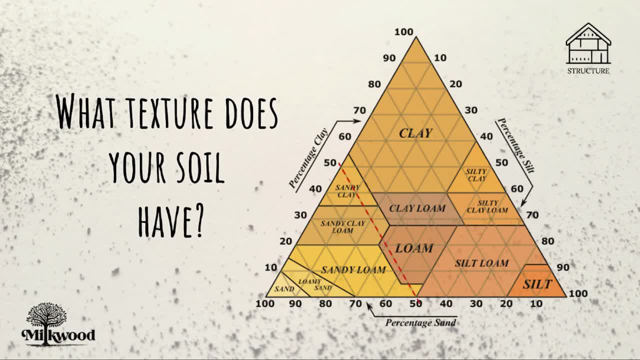 So in our example we've got 50 percent sand. you know, here's the sand axis and it goes up at this angle. so 50 percent sand and we had 15 percent clay. so this is the clay axis and it's horizontal, so you just go across here and where they cross. 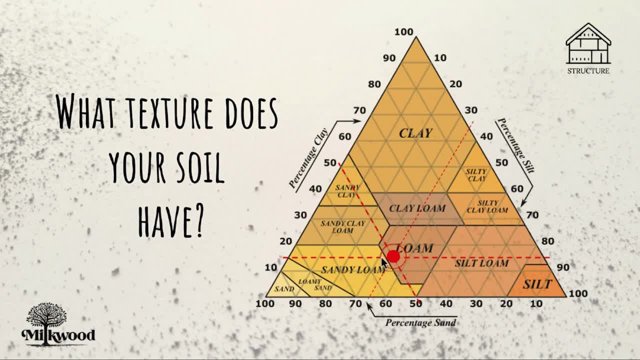 that's what type of soil texture you've got. In this case, in our example, we've got a loamy soil, a lovely loamy, equal sort of soil. it's not too heavy in clay, it's not too sandy, it's not too silty, it's right in the middle. 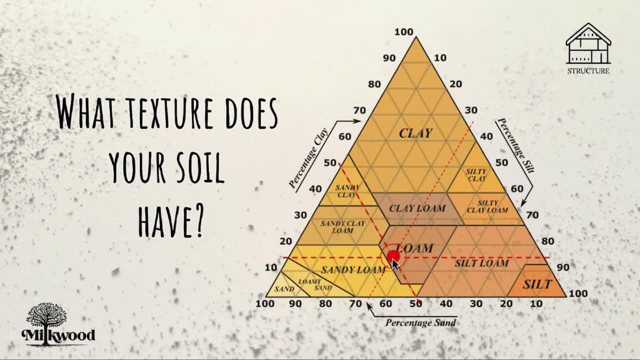 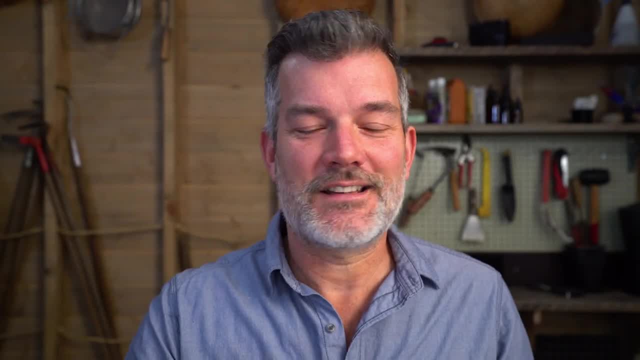 We don't even need to calculate the 35 percent, because it can't be anything else. So, bingo, we have a loam soil, lucky us. If your numbers aren't as neat as ours- and they won't be- then this can be a little complex to work out. So we've made 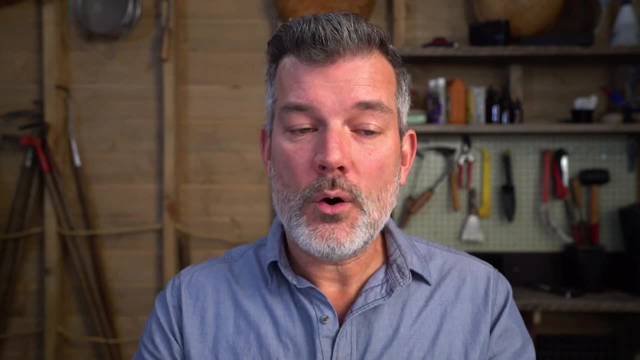 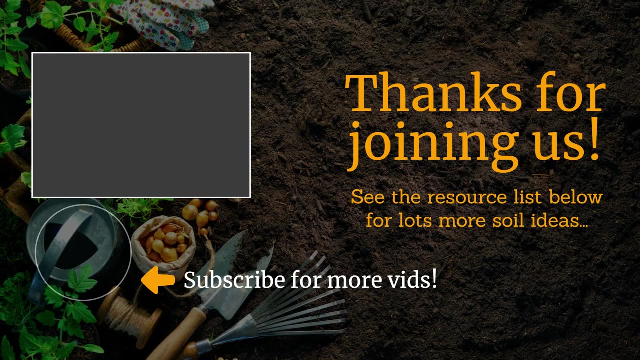 a handy little online calculator where all you have to do is enter in the heights of each of the different layers and it plots your soil texture on this scale. and you're good to go.